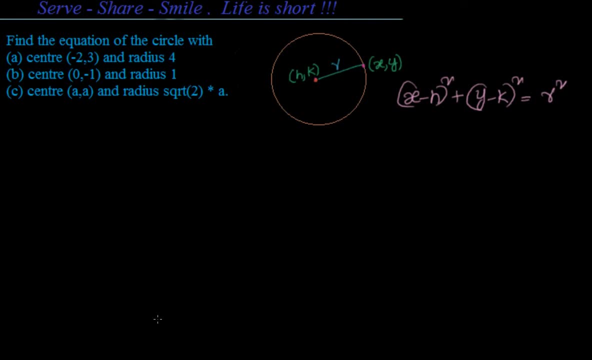 then we know that the equation of the circle is given by x-h whole square plus y-k whole square, equal to r square. Now, in this session, let us try to leverage that formula and to do simple examples. So let us look at these examples. 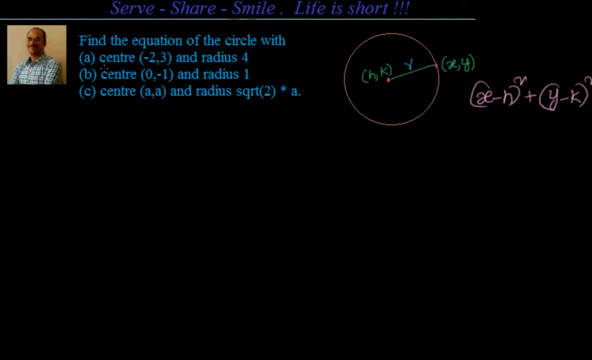 The first one we have to find out the equation of the circle given to us. that center is minus 2 comma 3.. So can I say h equal to minus 2, k equal to 3 and radius r equal to 4.. 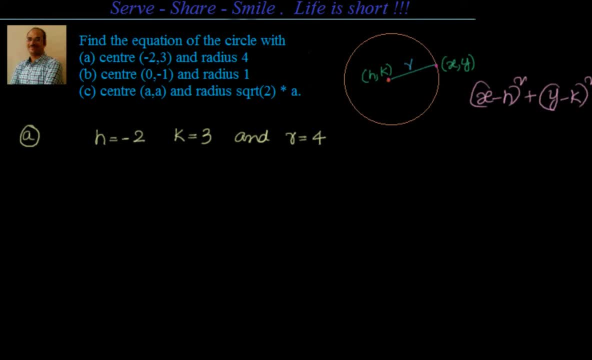 We know the equation, So I will directly go ahead and substitute in the equation. Let me write the equation here: x-h whole square plus y-k whole square equal to r square. Now if I substitute the values, I will have x minus half, h is minus 2.. 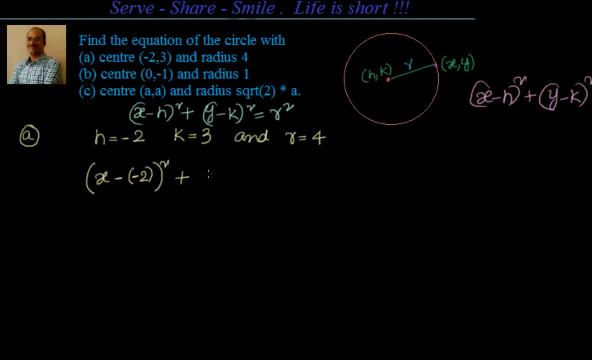 So that will be x minus minus 2 whole square. plus y, k is 3.. So y minus 3 whole square equal to r square. That is equal to 4 square. If you simplify this, this will be nothing but x plus 2 whole square plus y minus 3 whole square, equal to 4 square. 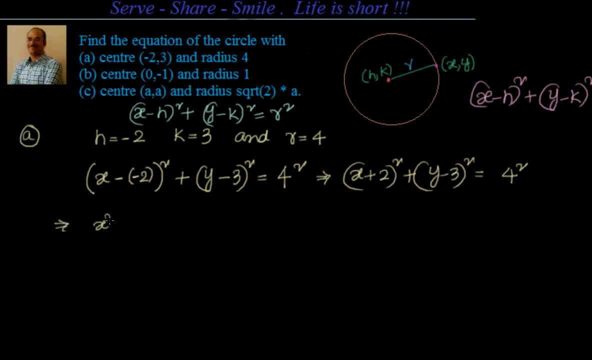 We can expand that and simplify. We will have x square plus 4x plus 4.. It is in the form of a plus b whole square. Next term is in the form of a minus b whole square. So we will have y square minus 6y plus 9, equal to 16, which is nothing but equal to x square plus y square plus 4x minus 6y. 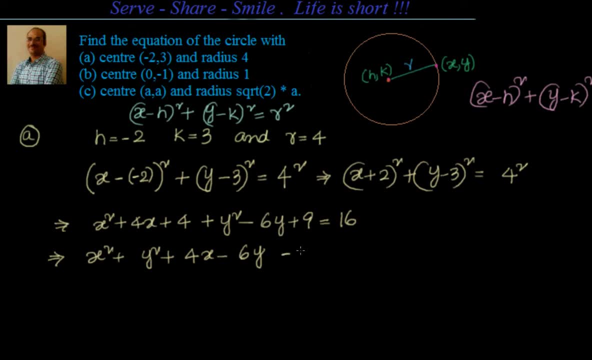 4 plus 9 is 13.. 16 is on the other side, So when it comes here you will have 0.. So it will be x square plus y square Plus 4x minus 6y. 4 plus 9 is 13.. 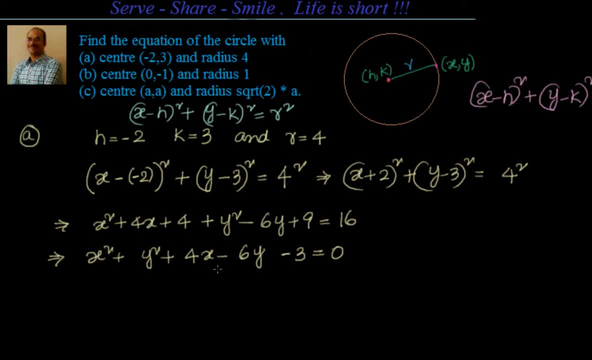 13 minus 16 is minus 3.. So x square plus y square plus 4x minus 6y minus 3, equal to 0, is the standard form equation of the circle. So let us do the next problem. So let us do the next one. 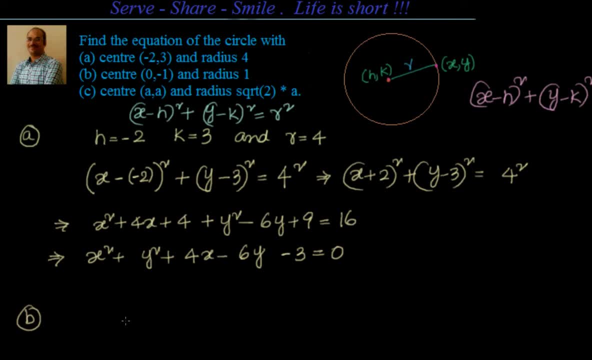 Let us do the next one. We have to find out the equation of the circle with center 0, comma of minus 1.. That means h is 0, k is minus 1 and we have been given radius is equal to 1.. 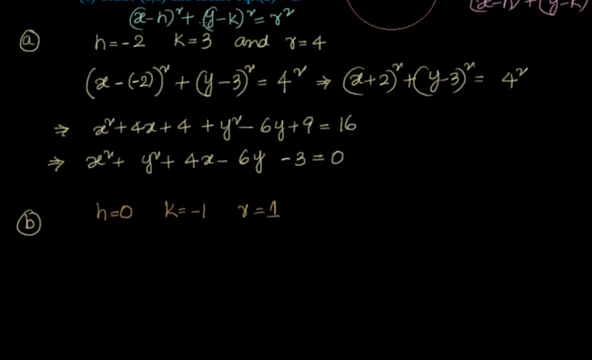 So what is the equation We have to substitute in: x minus h, whole square plus y minus k, whole square equal to r square. Very simple, direct substitution. So I will have x minus 0.. h, whole square plus y minus minus 1, because k is minus 1 whole square equal to r square. 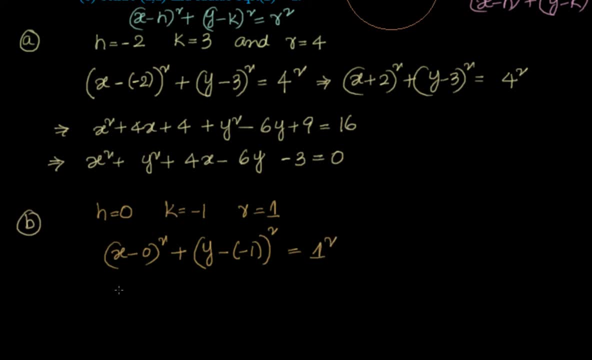 That is equal to 1 square. So if you simplify that, next step will be x square plus y plus 1, whole square equal to 1.. r, that is also equal to x, x square plus y square plus 2y plus 1, equal to 1, or x square plus y square plus 2y, equal to 0.. 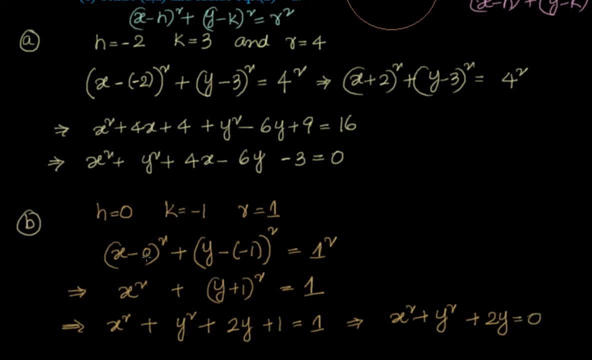 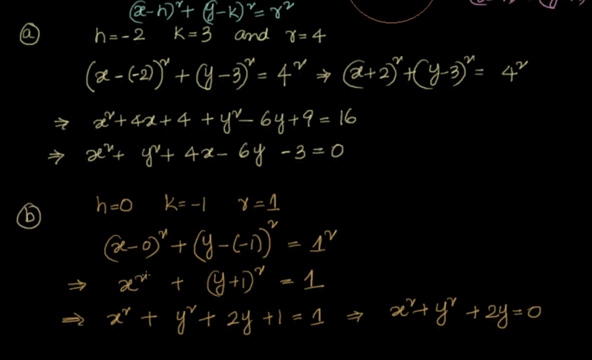 Let us check that again. We have h equal to 0, k equal to minus 1.. We have been given center 0 comma minus 1. And radius equal to 1.. So h equal to 0, k equal to minus 1,, radius equal to 1.. 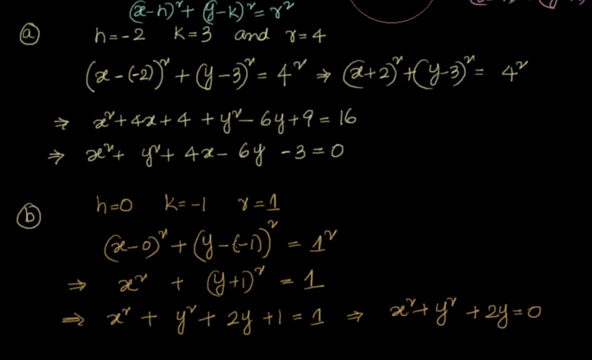 The formula is: x minus h- whole square plus y minus k- whole square equal to r. square x square plus y plus 1, whole square equal to 1, or x square plus y square plus 2y plus 1 equal to 1.. When 1 cancels, you will have x square plus y square plus 2y. 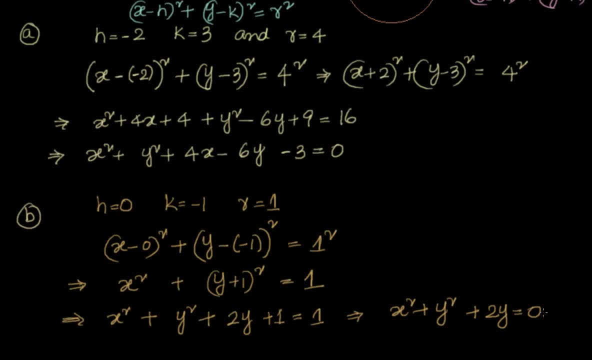 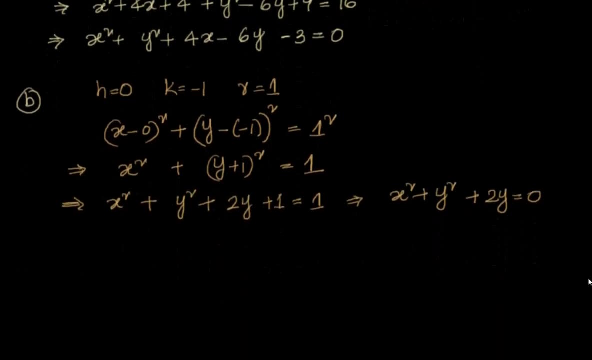 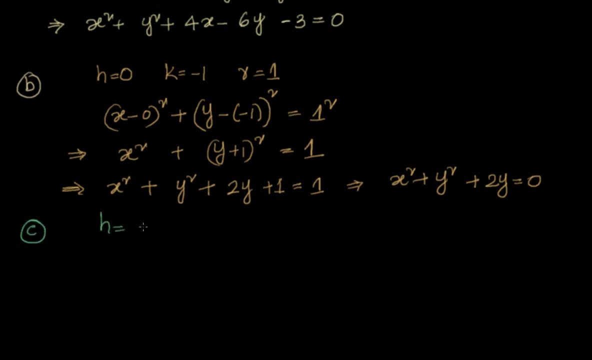 So x square plus y square plus 2y, equal to 0.. Let us do one more problem, The last one: Center, a comma a, radius root 2a. Let us do that one. So we have h equal to a because center coordinates are a comma a. 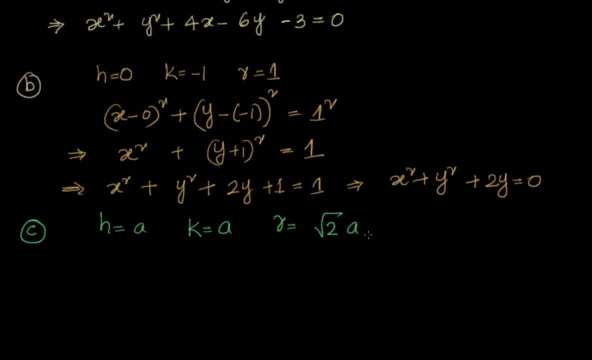 And radius equal to square root of 2 into a. So same formula: x minus h equal to 1.. Now we have h whole square plus y minus h, a whole square plus y minus k, whole square k equal to a here. 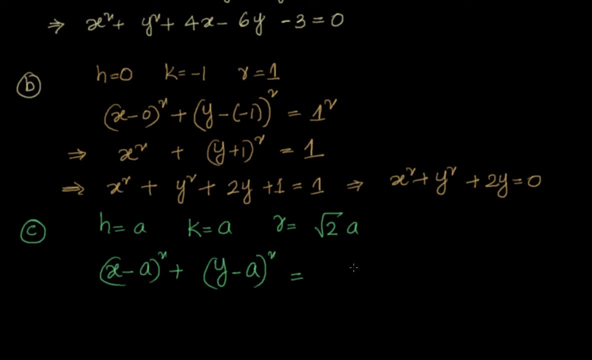 So it is x minus a whole square plus y minus a whole square equal to r square. That is root 2a whole square. So that's nothing but equal to x square minus 2ax plus a square. I am just substituting the formula a minus b whole square equal to a square minus 2ab plus b square, which you should be very comfortable. y square minus 2ay plus a square. y square minus 2ay plus a square. that is y minus a whole square equal to root 2 whole square is 2. a whole square is a square. 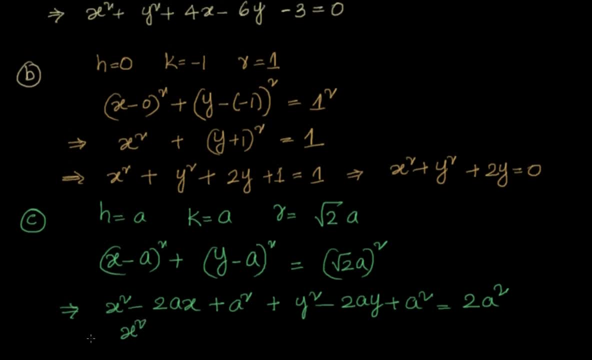 So the next step will be x square plus y square, minus 2ax minus 2ay, equal to 0, because a square plus a square is 2a square, 2a square, 2a square cancels out. We are left with x square plus y square, minus 2ax minus 2ay, equal to 0.. So the next step will be x square plus y square minus 2ax minus 2ay, equal to 0, because a square plus a square is 2a square 2a square 2a square cancels out. So the next step will be x square plus y square minus 2ax minus 2ay, equal to 0, because a square plus a square is 2a square 2a square 2a square cancels out. 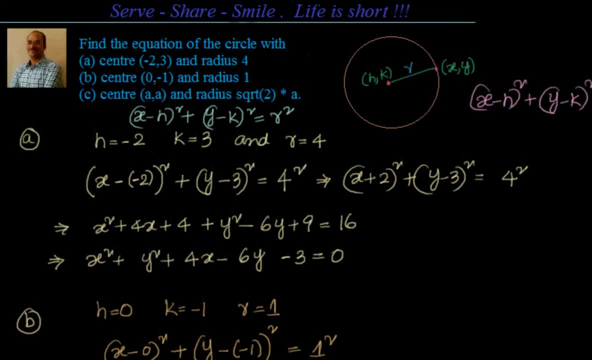 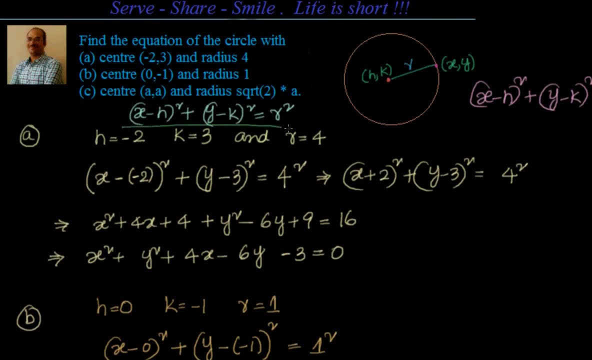 So in this way you can solve simple problems. If you have been given the coordinates of the center and you know the radius, then you can leverage the formula x minus h- whole square plus y minus k whole square equal to r square- That is the standard form of the circle- and find: 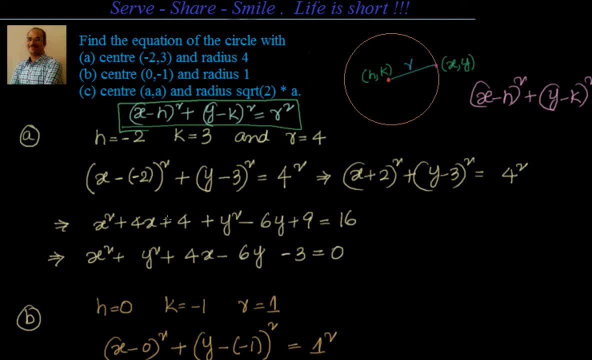 out the equation of the circle. In the next session what we will see is we have the equation from the equation: how to find out the center and radius. That is what we will see in the next session. So thanks for your time. I will catch you again in the next session. Bye for now.